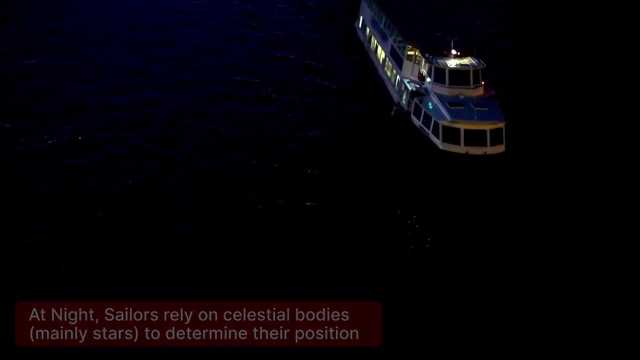 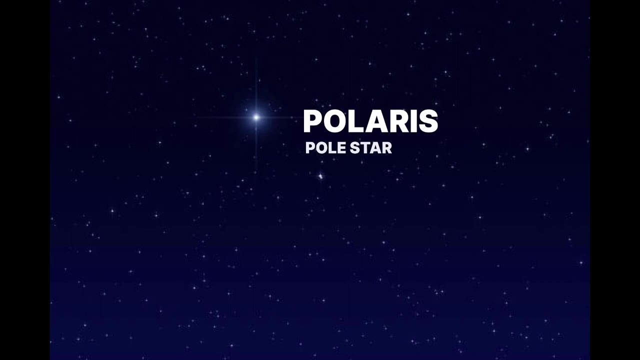 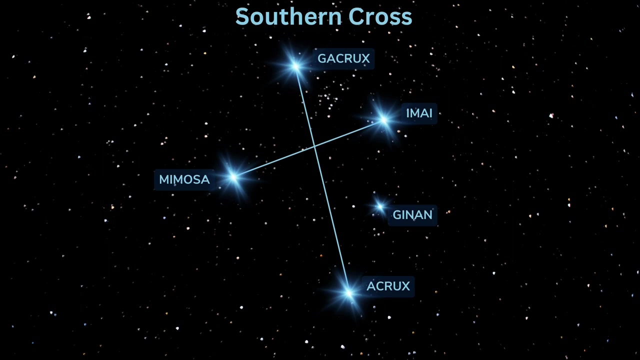 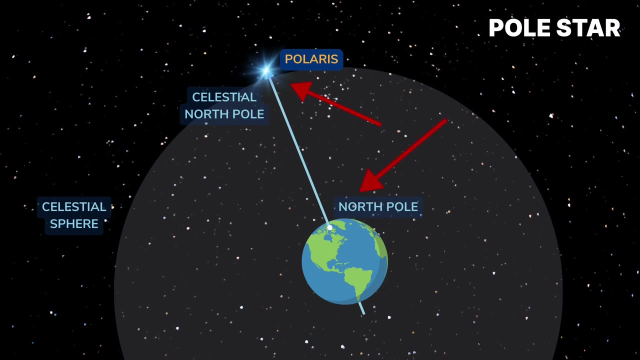 stars to determine their position and course at sea. The key celestial bodies used in navigation are Polaris, also called the Pole Star or the Nautilus star in the Northern Hemisphere, and the Southern Cross in the Southern Hemisphere. The pole star is located very close to the celestial North Pole, which is the point directly. 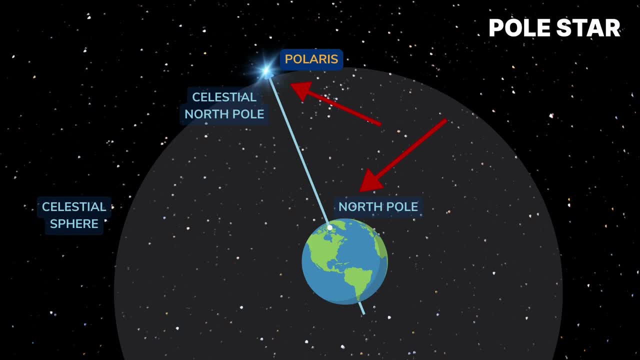 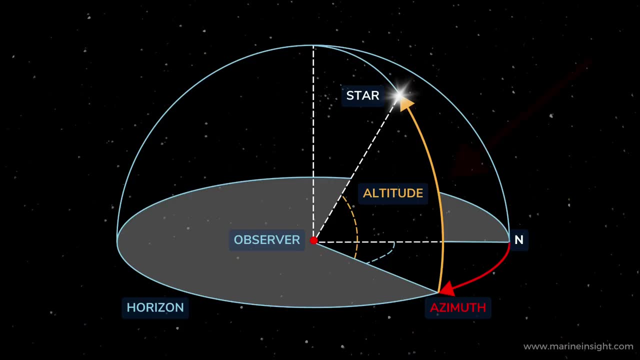 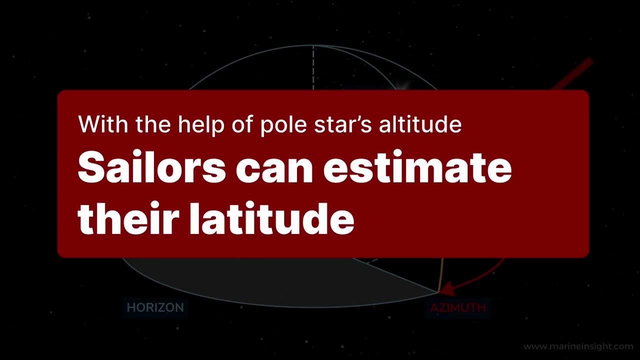 above the geographic North Pole of the Earth. It serves as a reliable and constant reference point in the night sky for sailors in the Northern Hemisphere. By observing the angle between the horizon and the pole star, known as the star's altitude, sailors can estimate their latitude. 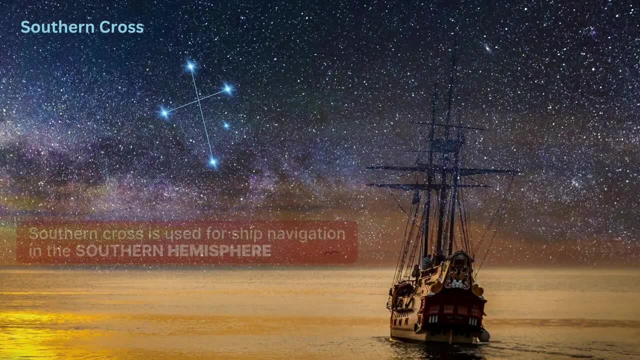 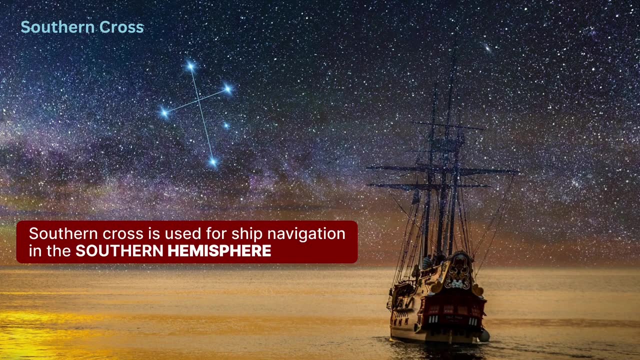 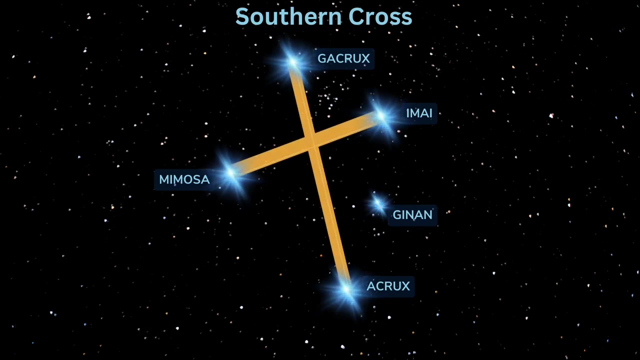 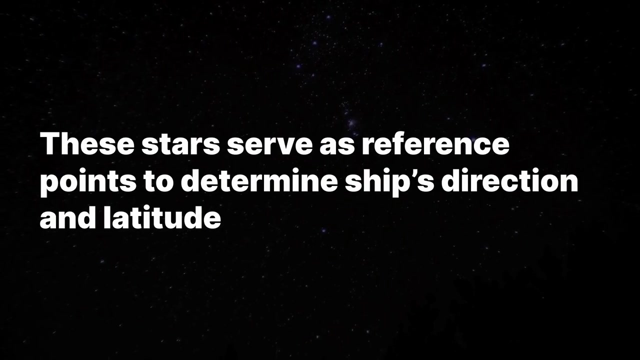 The Southern Cross, also known as Crux, is used for ship navigation, primarily in the Southern Hemisphere. It serves as a prominent celestial reference point. It is a distinctive and easily recognizable constellation consisting of four main stars that form a cross shape. These are certain stars that serve as reliable reference points for determining the ship's. 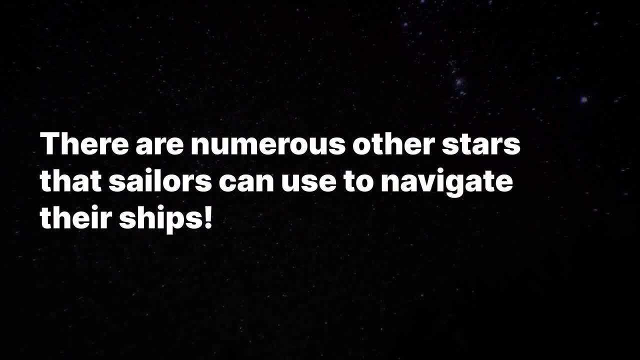 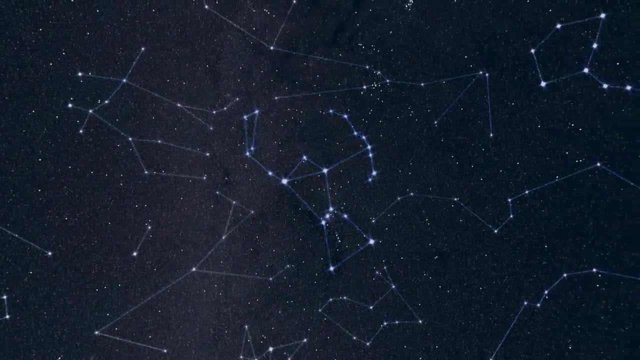 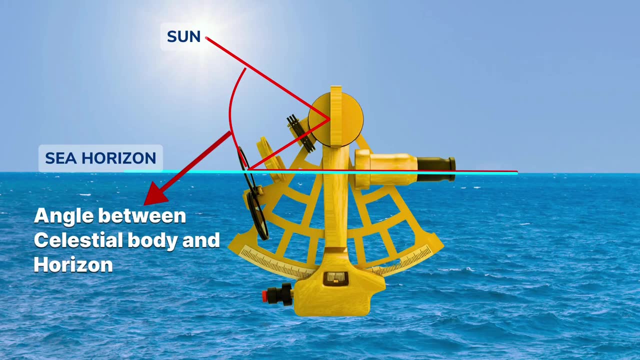 direction and direction. There are numerous other stars as well that sailors use to navigate their ships. To navigate by the stars, sailors use an instrument called a sextant. The sextant allows them to measure the angle between a celestial body, usually the sun. 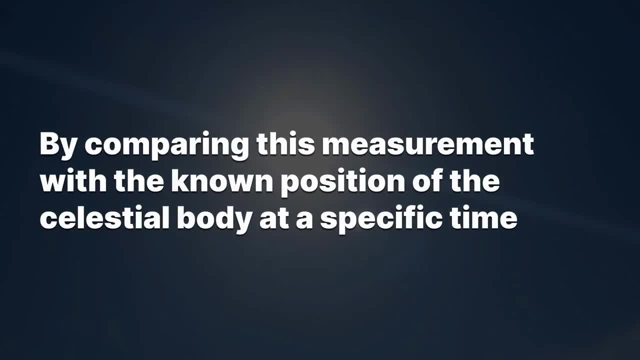 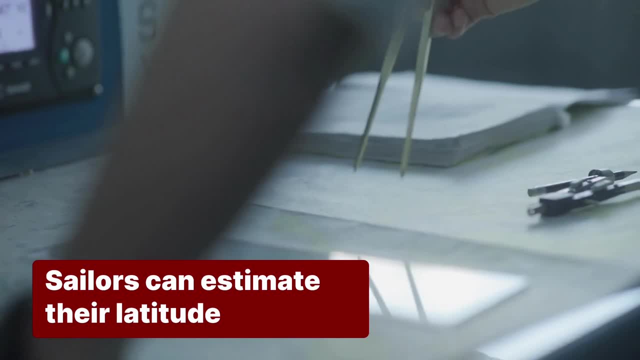 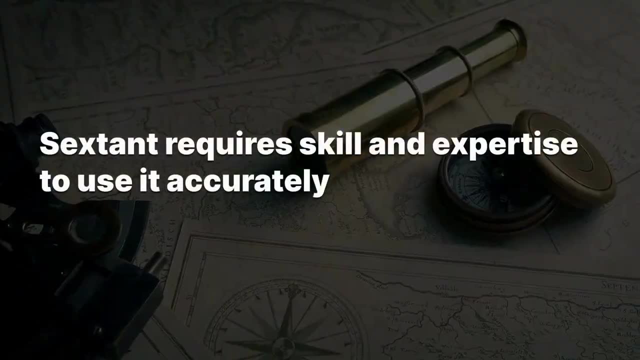 or a star and the horizon. By comparing this measurement with the known position of the celestial body at a specific time, sailors can calculate their latitude and latitude. The sextant measures the angle between the celestial body and the horizon. The sextant measures the altitude, namely the position of the stars above the horizon. 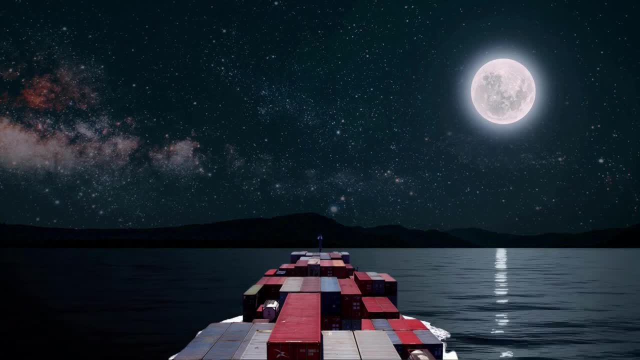 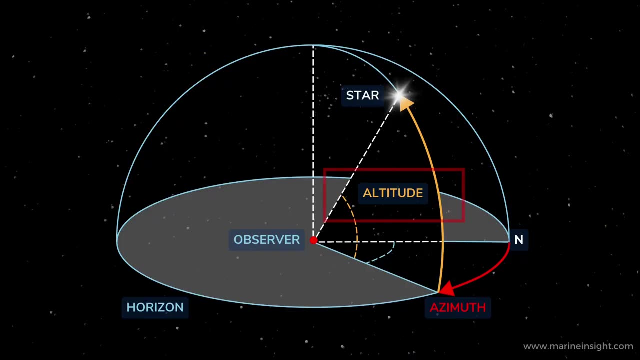 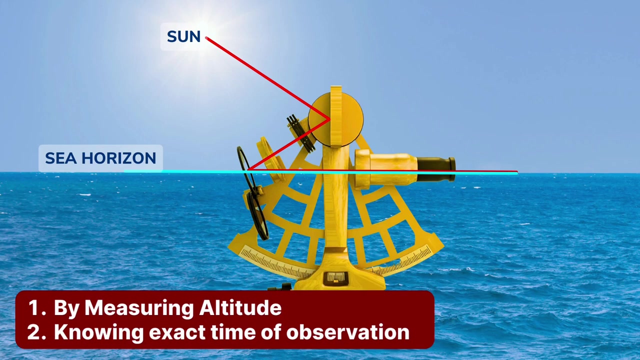 Navigating by the stars also involves understanding various celestial navigation concepts. One such concept is the altitude of a celestial body, which is the angle it appears above the horizon. By measuring the altitude and knowing the exact time of the observation, sailors can plot their position on the star. 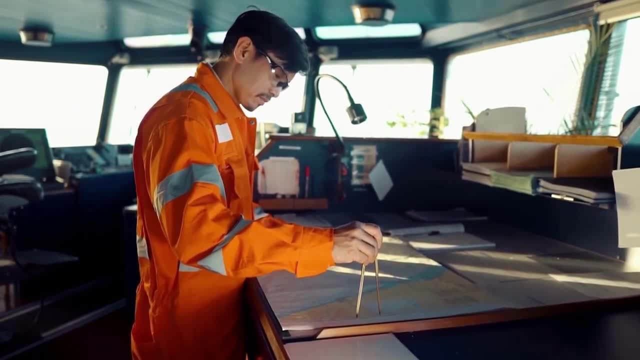 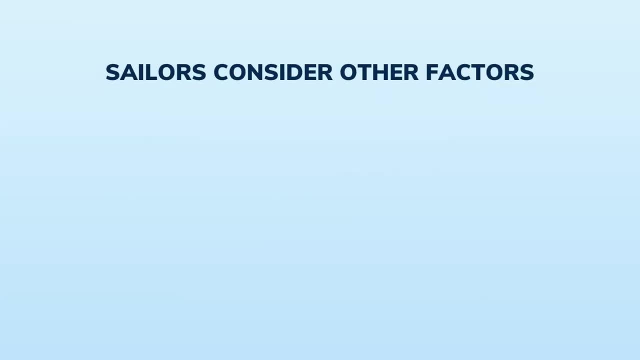 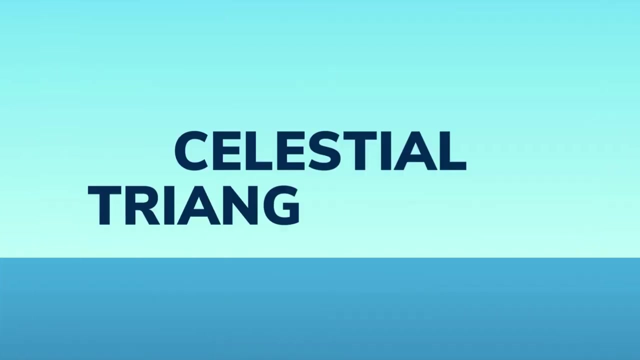 a nautical chart using special navigation tables and mathematical calculations. additionally, sailors consider other factors such as the ship's speed, course and time to determine their position accurately. they take multiple celestial sightings over time to establish a reliable fix. this process is known as celestial triangulation, where intersecting lines are drawn.